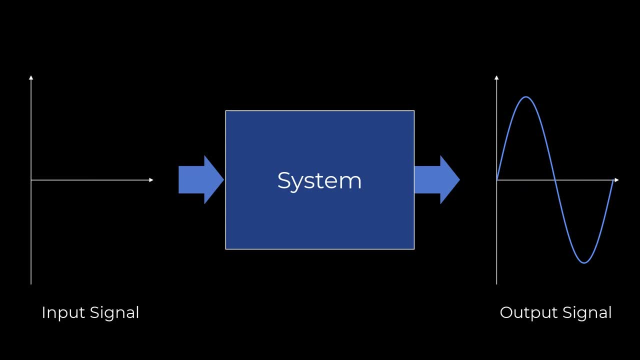 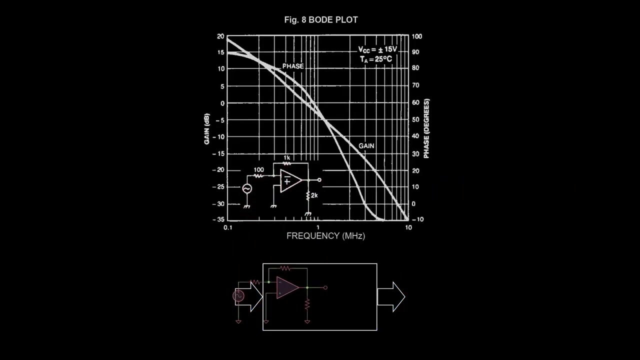 passing through a system. But there's more. The Bode plot doesn't illustrate how just one signal changes, but how signals of various frequencies are affected. The Bode diagram gain plot depicts how the magnitude of signals change as they pass through the system. 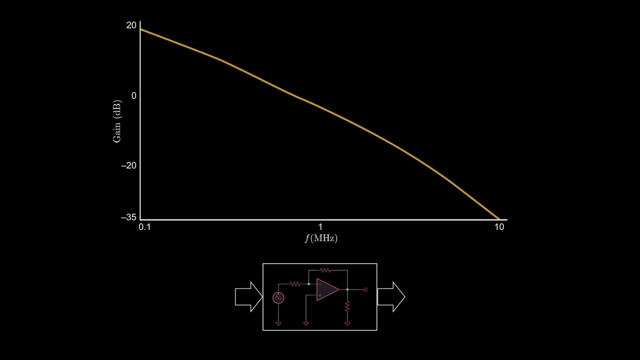 In this op-amp circuit, low frequencies are amplified. At 100 kHz, signals are amplified by nearly 20 decibels. That's an amplification of 100 times. At higher frequencies, the gain diminishes. At a frequency of 300 kHz, the gain drops. 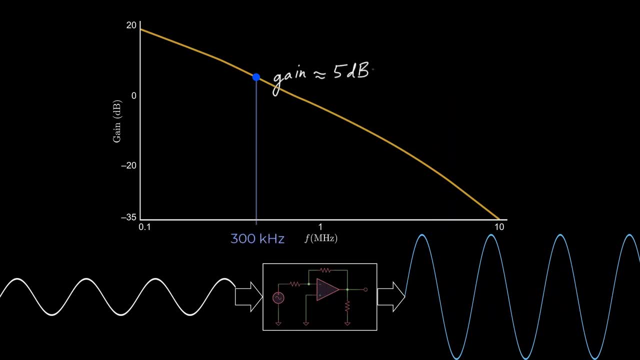 to 0.. At higher frequencies, the gain diminishes. At a frequency of 300 kHz, the gain drops to 5 dB, equivalent to an amplitude multiplier of about 3.2.. This trend continues and we reach 0 dB at about 700 kHz, implying no gain or loss in the signal. 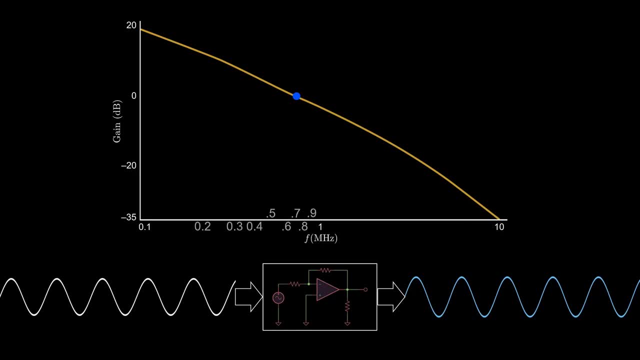 Notice that both the frequency and gain axes are logarithmic. This is typical in a Bode diagram. The logarithmic axes can be confusing but make a broad range of frequencies and gains intelligible from a single graph. Look how difficult it is to read the high frequency behavior from the same data plotted. 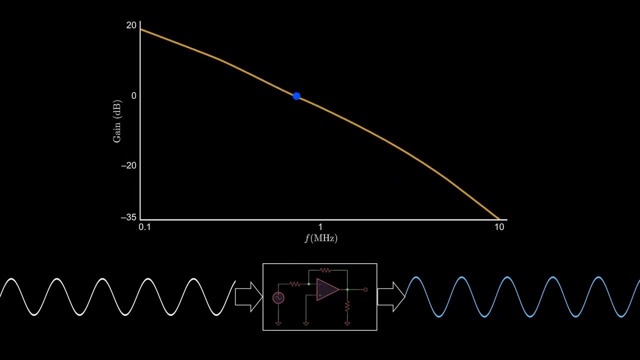 on linear axes At high frequencies this op-amp feedback circuit doesn't even produce a gain. Signals lose, amplitude diminishing by 20 dB at 4 MHz. That's a hundred-fold amplitude loss. Often we're mainly interested in the gain plot, But let's not forget that the gain is. 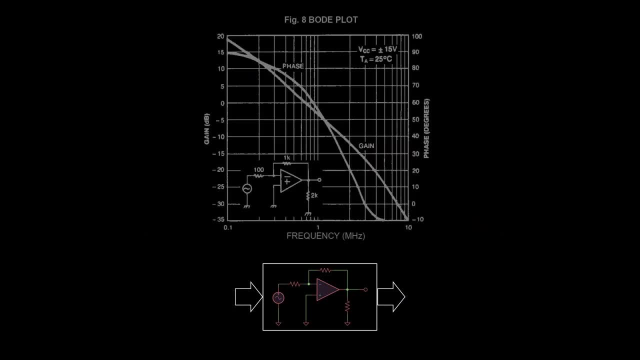 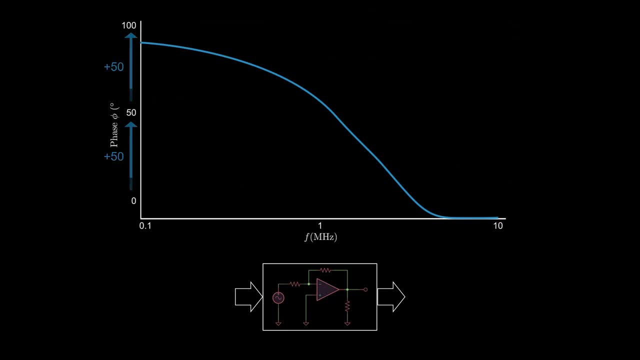 This is an example of the gain and this is the base of the gain. This is a good example of the gain as it is applied in this diagram, But we need to not forget about the phase. Unlike the gain, the vertical axis of the phase plot is linear, but is plotted against. 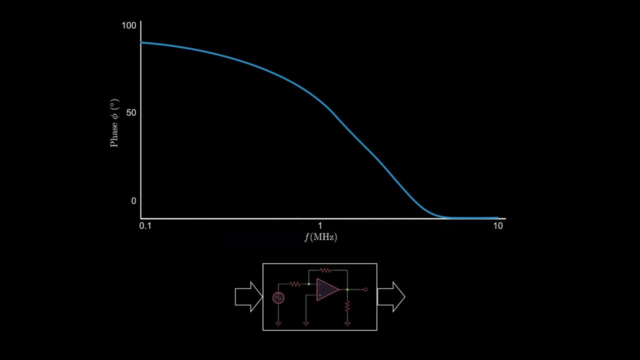 the same logarithmic frequency axis For this op-amp circuit there's a 90 degree phase shift at 100 kHz. That means the output signal is offset from the input signal by one-fourth the period to the left. Note that I'm ignoring the gain characteristics to simplify the illustration. 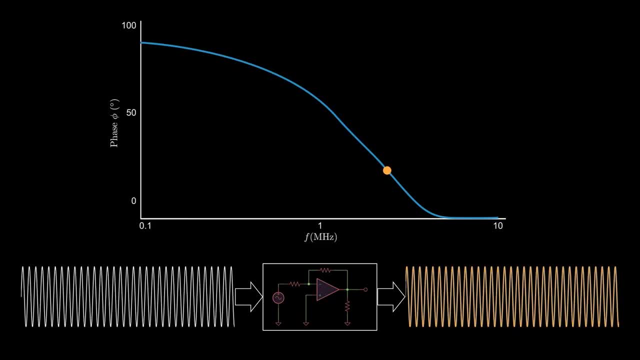 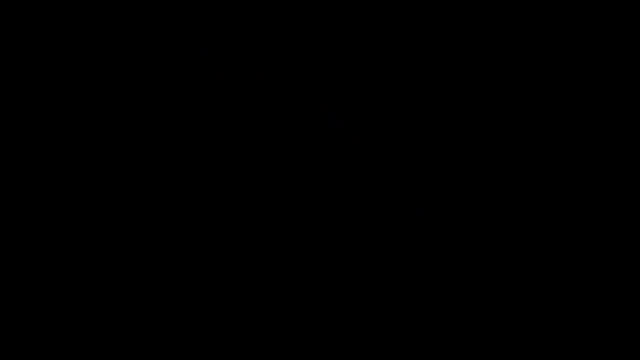 As frequencies increase, the phase approaches zero At 3 MHz. the input and output signals are in phase. If you're interested in Bode plots, you're probably already familiar with the Fourier transform. You can use a Fourier transform to calculate the frequency content of a signal. 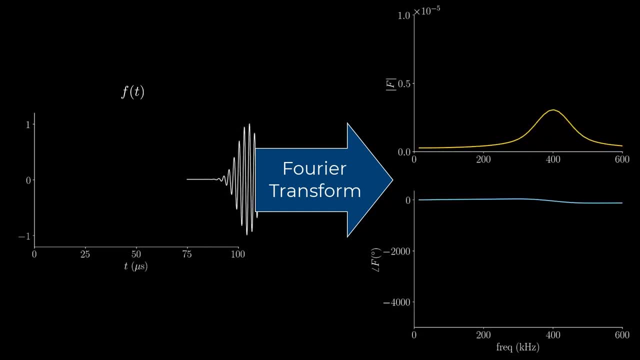 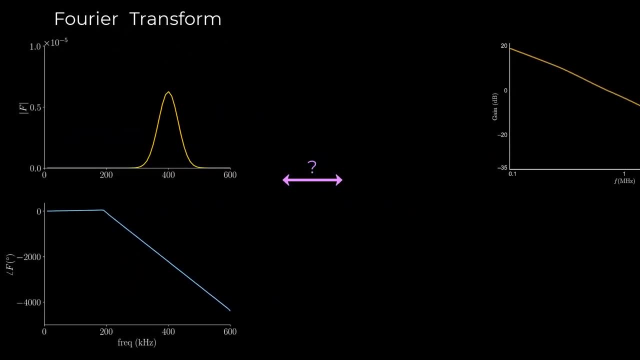 A common way to plot the frequency content of a signal is using magnitude and phase plots. But you might wonder: how are these different from the gain and phase plots of the Bode diagram? Let's return to our op-amp example. An input signal V in is applied to the circuit. 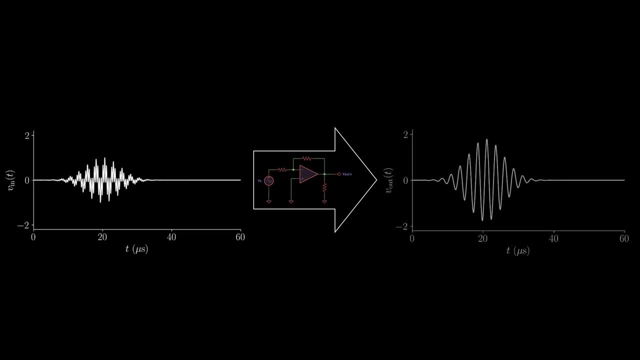 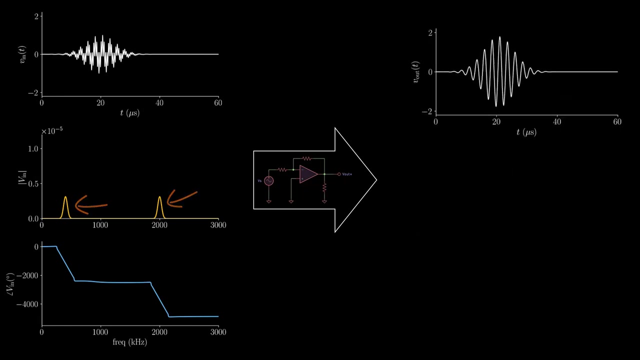 The op-amp amplifies the signal, resulting in V out. The frequency content of the input signal can be analyzed by plotting the magnitude and phase of its Fourier transform. This input signal has peaks at 400 kHz and 2 MHz. The output signal shares the 400 kHz peak, but the 2 MHz peak has diminished. 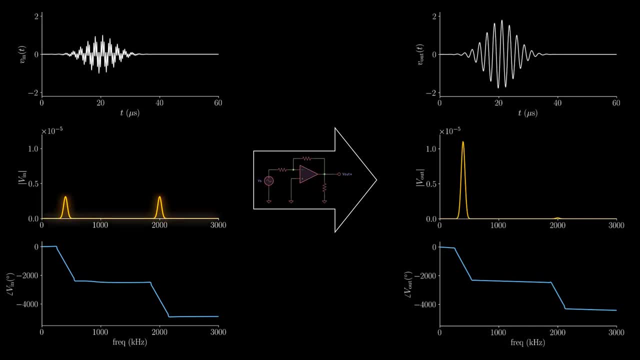 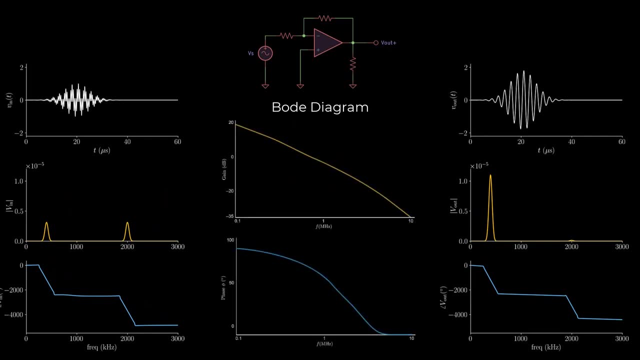 This is a typical use of the Fourier transform to compare the frequency content of signals. The Bode diagram, on the other hand, doesn't characterize individual signals. Instead, it illustrates the relationship between input and output signals of a given system. At 400 kHz, the Bode diagram shows an amplification. 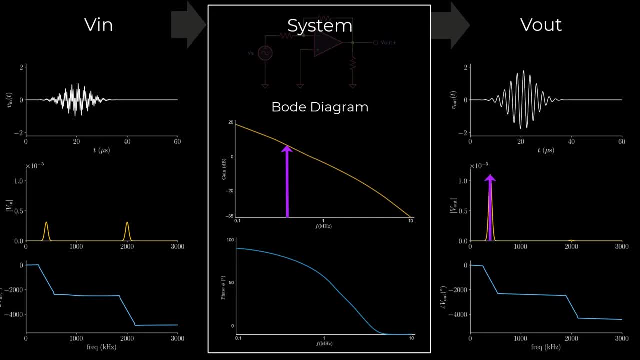 This is what we observed in the frequency content of the output signal. Overall, this Bode diagram illustrates that low frequencies are amplified, while high frequencies are attenuated. Compare the Fourier magnitude plots of the input and output signals. The Bode diagram shows that the input and output signals are amplified, while the high 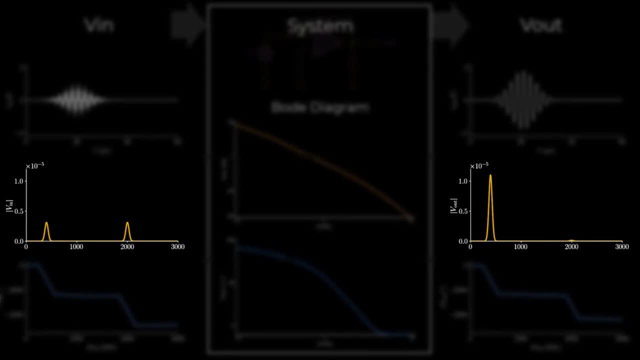 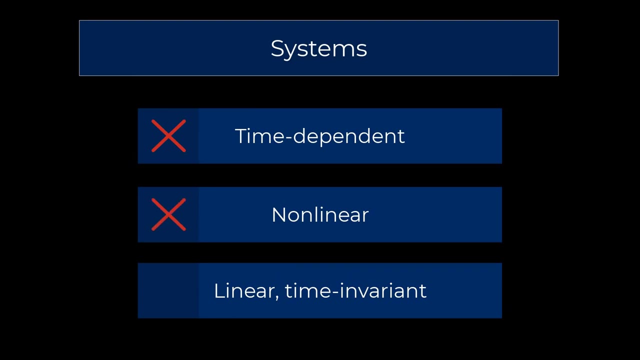 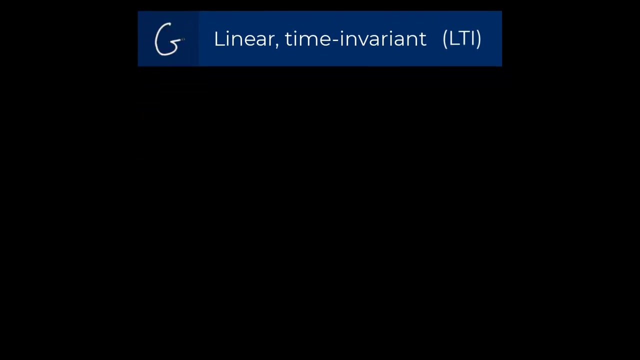 frequencies are at 400 kHz, You'll notice changes here. It's worth noting here that Bode diagrams aren't valid for any system. They're only valid for linear time-invariance systems, usually abbreviated LTI. A linear system requires that the effect of the system applied to separate signals is 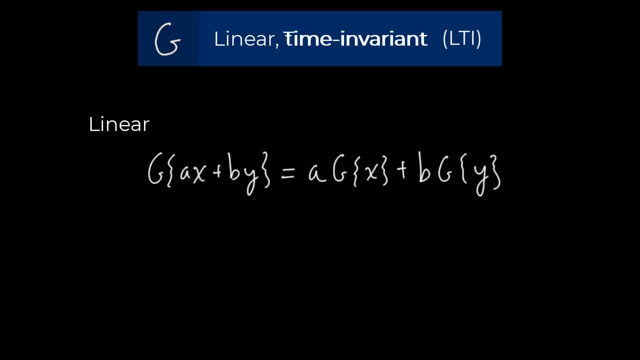 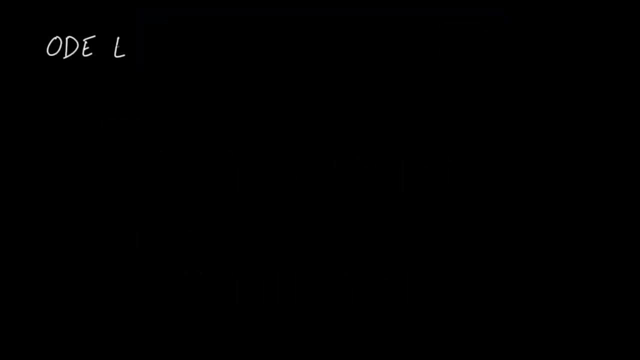 equivalent to the linear combination of the signals affected separately. Time invariance requires that the effect system on an equal input signal at a later time will be the same. So how do you know if your system is LTI? Usually it's because you've written the differential equation for your system and 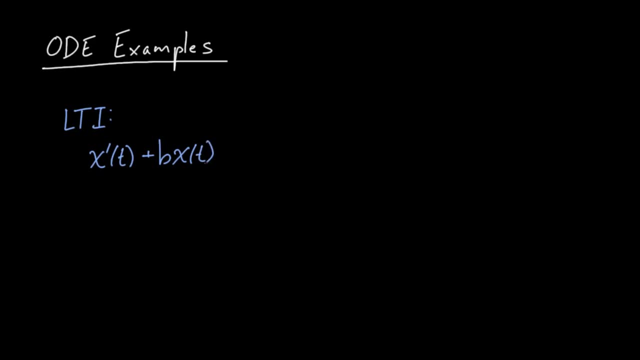 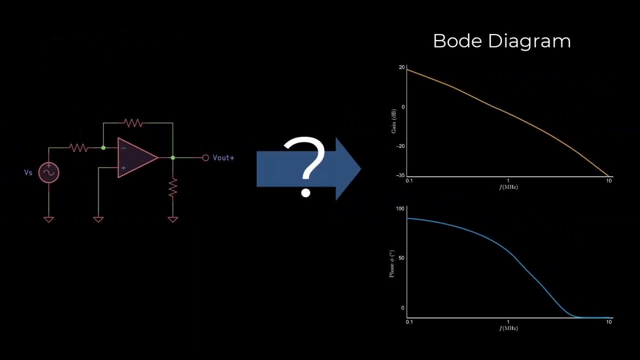 it's linear and has no explicit time dependence. Here's a couple examples of non-LTI systems. Explicit time dependence: in sine of t Non-linear cubic term in x of t cubed. You can't really understand a Bode plot until you know how it was created. 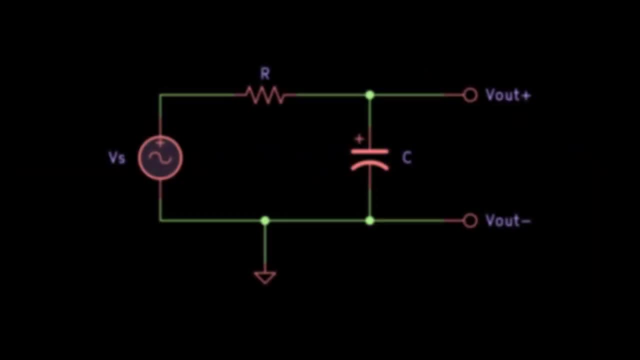 In this chapter of the video, I'll build up the Bode diagram for this RC circuit starting from scratch. This will involve some math, but don't worry, I'll walk you through the steps. Let's start by deriving the ODE circuit. 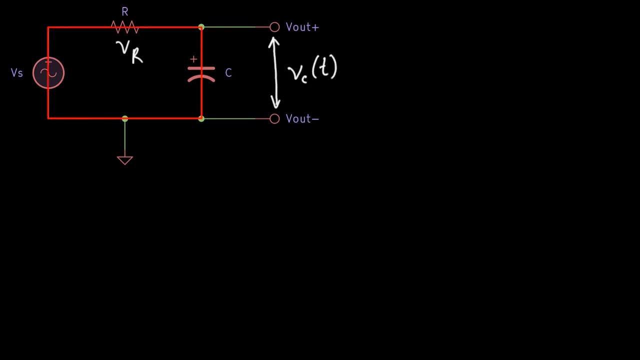 Let's start by deriving the ODE circuit for the output voltage. Kirchhoff's voltage law tells us that the net voltage around the closed loop will be zero. We're interested in the voltage drop across the capacitor because that gives our output voltage. so we want to write everything in terms of Vc. 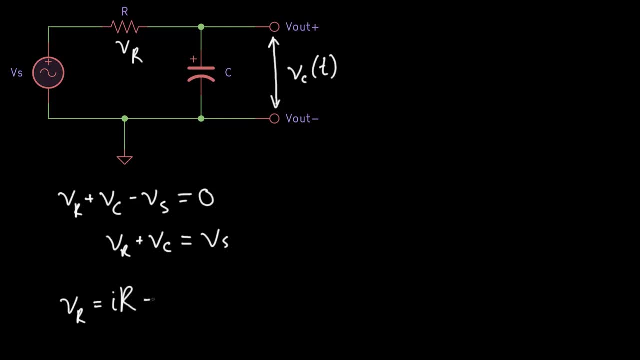 Using the relationship between voltage and current in a capacitor and the fact that the current is constant. in this simple circuit, we can rewrite the voltage across the resistor in terms of Vc. We don't need to rewrite Vs because we're assuming it's an arbitrary input voltage. 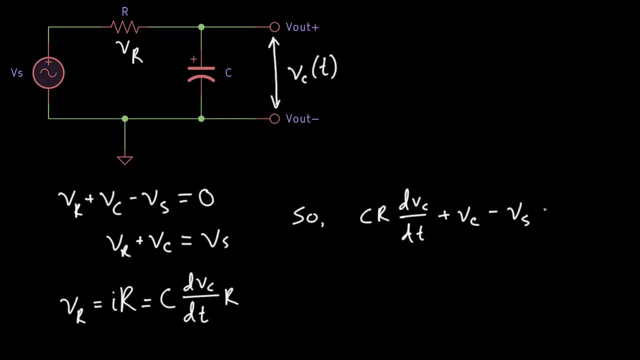 signal unrelated to the dynamics of the RC filter. Let's look at a solution of this ODE, assuming an input sinusoid with a frequency of 10 Hz. If I was back in undergrad, I'd use my favorite technique with complex exponentials to solve. 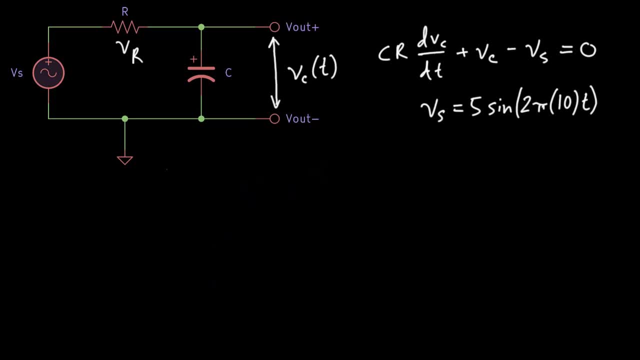 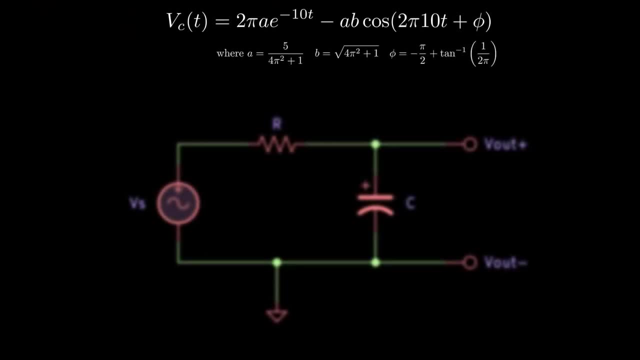 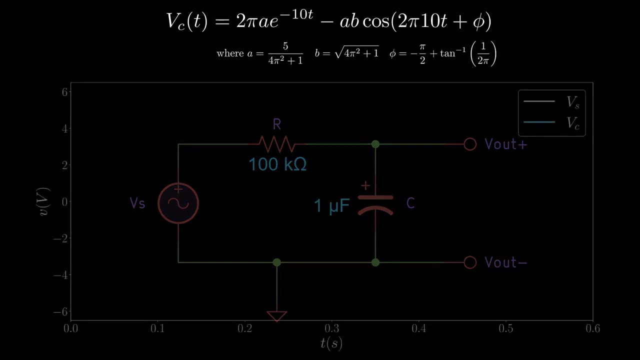 this, But this isn't a video about solving ODEs, so let me just write out the solution. I'm going to write out the solution. I've written the solution for an RC circuit with a 100kΩ resistor and a 1uF capacitor. 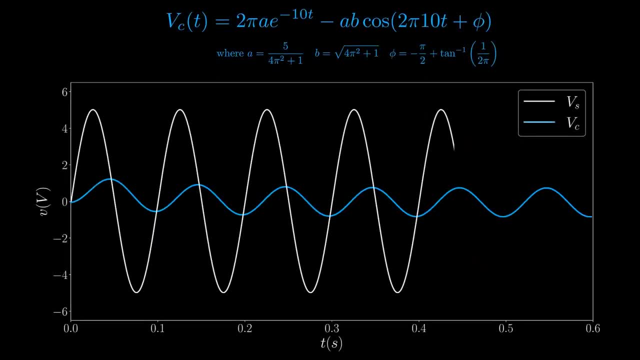 If we plot the solution Vc and the input signal Vs, we'll notice that the magnitude has diminished and the phase has shifted. The phase shift of the sinusoid is approximately negative 81 degrees. The gain is around 1.5.. The phase shift of the sinusoid is approximately negative 81 degrees. 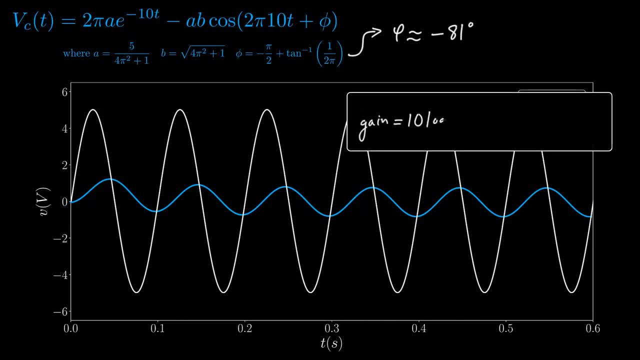 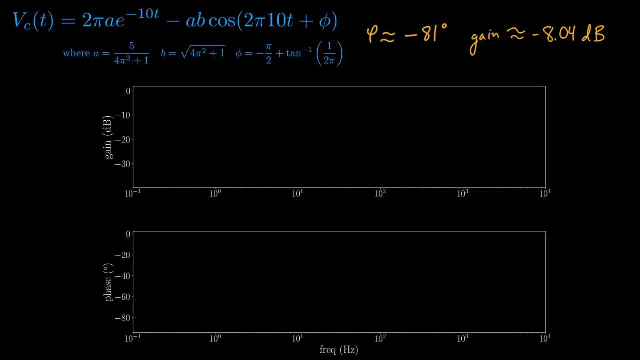 The gain is around 1.5.. The phase shift of the sinusoid is approximately negative 81 degrees. The gain is around 1.5.. The phase shift of the sinusoid is approximately negative 81 degrees. The of the long-term periodic behavior of this 10 Hz signal represent a single point in the Bode plot. 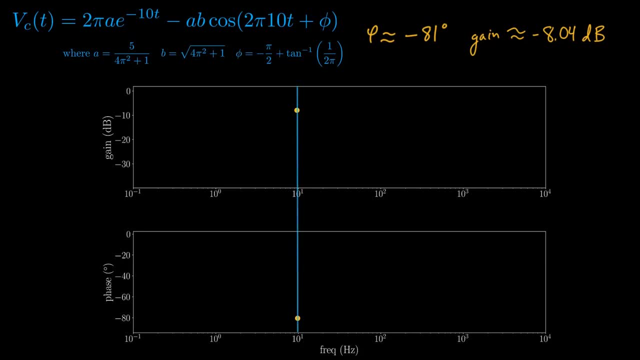 We could fill in the rest of the Bode plot by varying the input frequency and computing the phase and gain from the ODE solution. But there's actually a much cleaner way to construct the Bode diagram analytically. Let me show you. 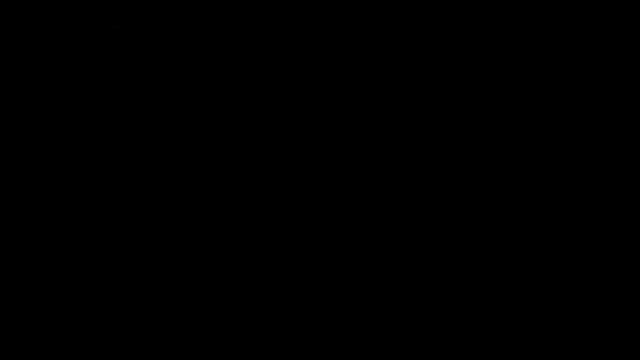 Transfer functions are a standard tool for analyzing LTI systems, like our RC circuit ODE. There are two steps to compute the transfer function. First we'll take the Laplace transform of the ODE. It sounds hard but there are simple rules for the Laplace transform. 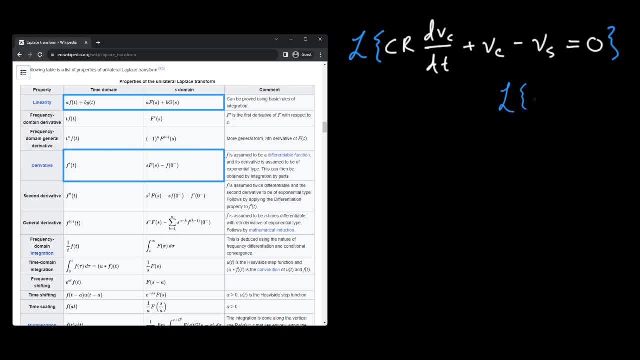 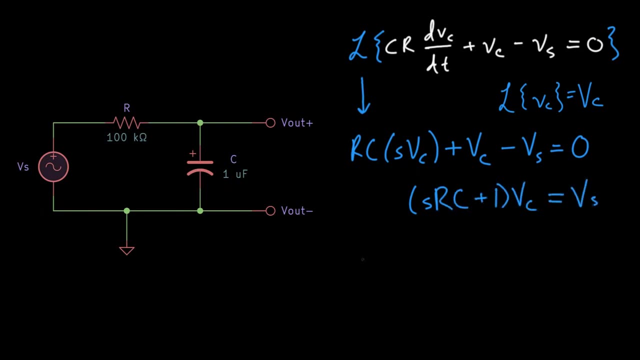 that you can find in a table. that makes it quite easy Applying these rules yields the Laplace domain form of the ODE. The transfer function is the ratio of the output signal Vc to the input signal Vs in the Laplace domain. A little algebra and we're there. 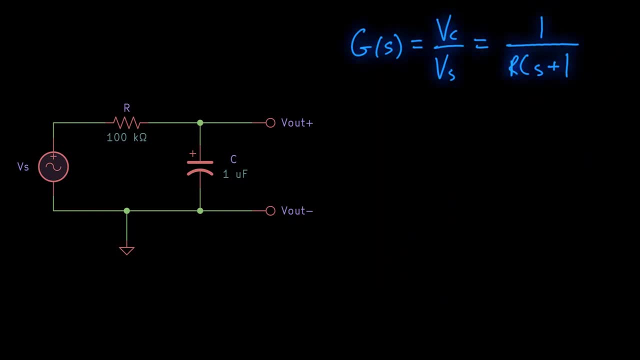 The RC circuit transfer function models both the transient and long-term behavior of the system. Restricting the Laplace domain independent variable s to its imaginary term Iω limits our analysis to the long-term periodic behavior. The gain is calculated by computing the magnitude of the complex transfer function. 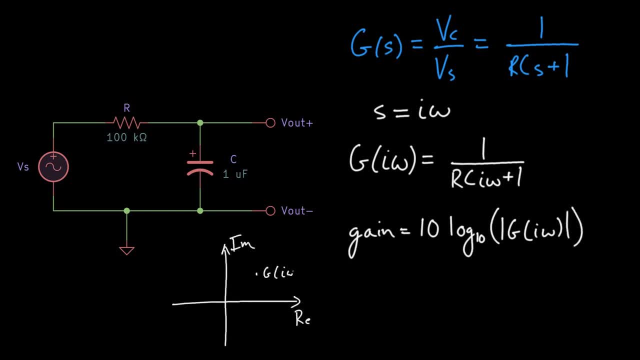 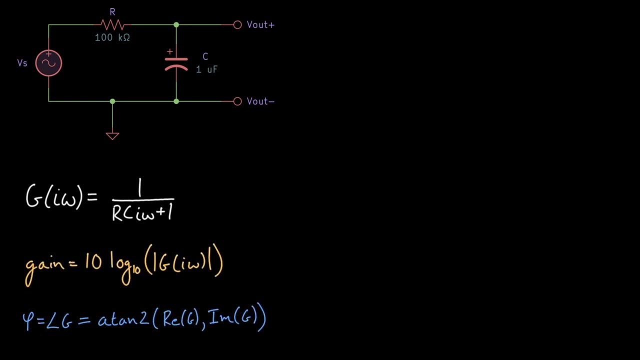 and then taking its log. The phase is the depicted angle in the complex plane. It can be computed using the arctangent. To construct the Bode diagram we simply plug in a range of frequencies and plot the resulting phase and gain. Here's the resulting Bode plot for this RC circuit. 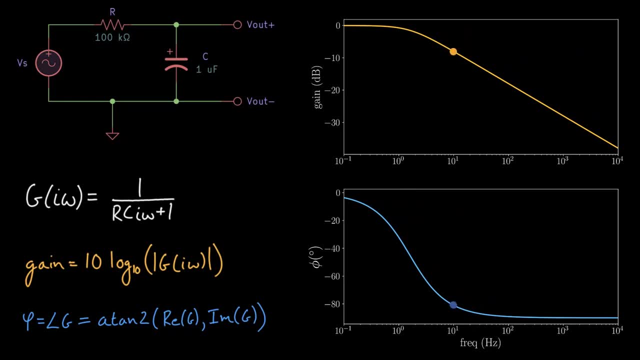 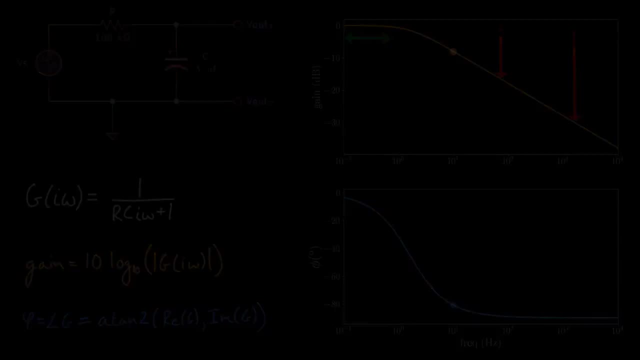 You can see that the ODE solution phase and gain are equal to the phase and gain calculated using the transfer function. This RC circuit is a low-pass filter because it attenuates high frequencies but allows low frequencies to pass. Here's another way you can create a Bode diagram. 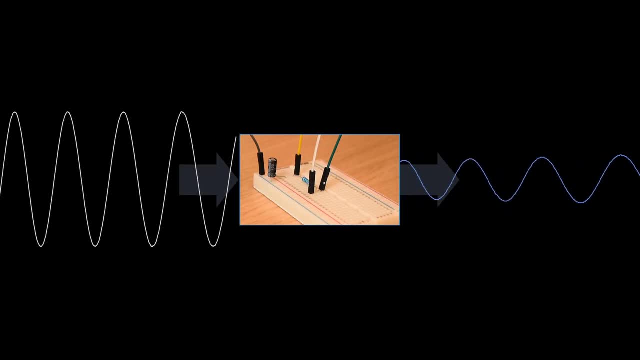 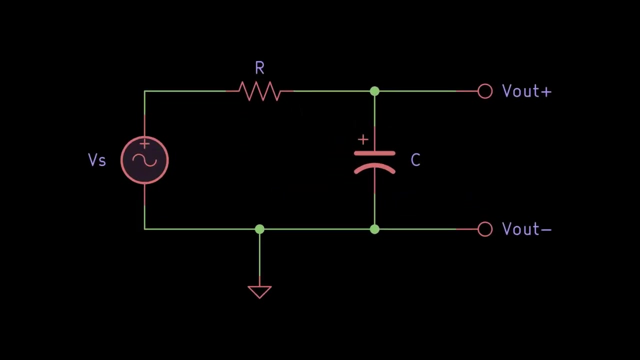 Probe a physical system with multiple frequencies. If you record the inputs and outputs, you can compute the frequency response and use the result to plot the Bode diagram: gain and phase. Here I've created an RC circuit with a 10 kilohm resistor and a 0.47 microfarad capacitor. 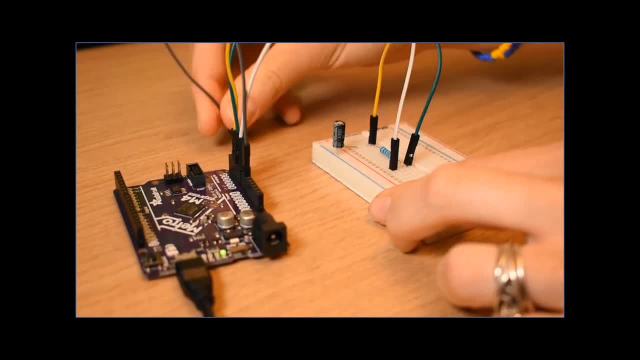 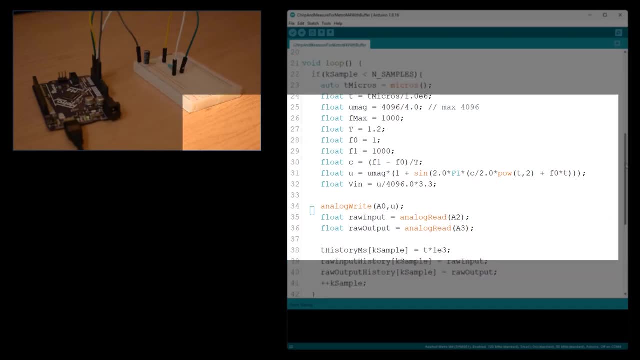 Here is the assembled circuit. Let's try probing the circuit with a chirp signal. I'll generate the chirp in the Arduino IDE. Here's the line where it's computed And here's where it's written to the digital-to-analog converter. 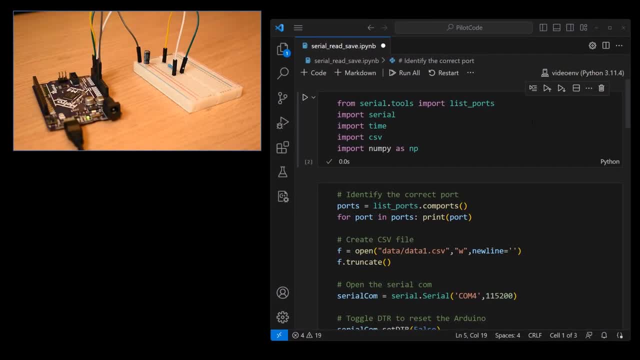 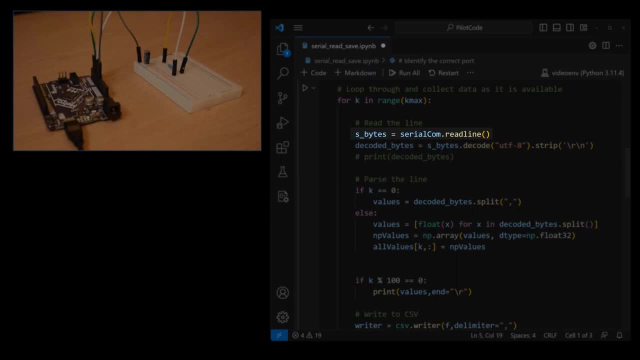 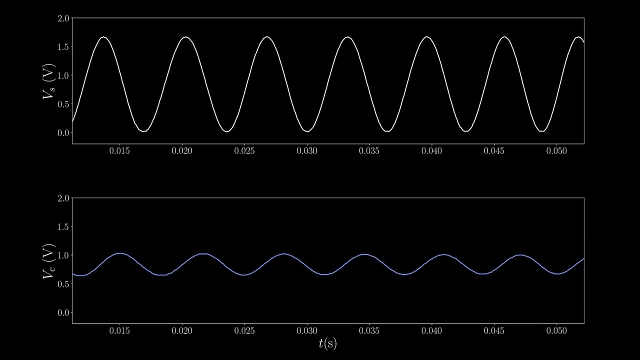 To record the inputs and outputs for processing, I'll use a simple Python script. Here's where we read from the serial port. Here's a video of the recorded input and output signals in a fixed time window. The input chirp signal starts at 1 Hz and ramps linearly to 1 kHz. 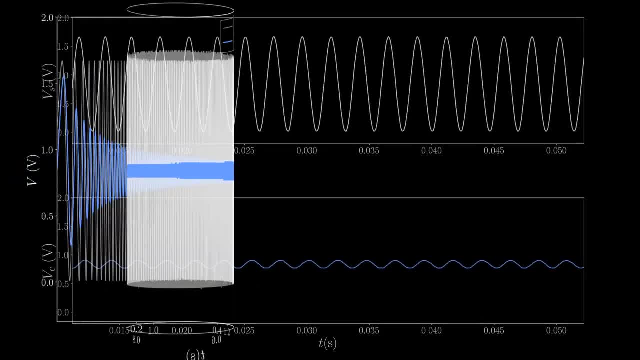 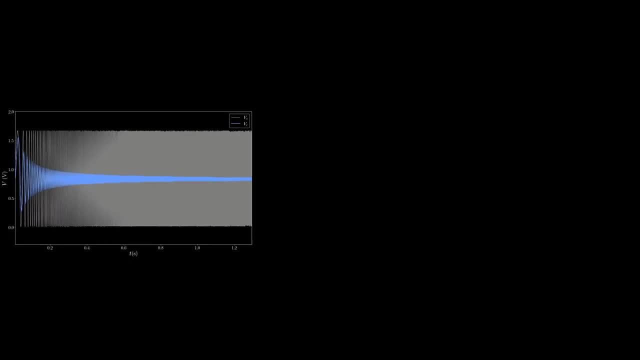 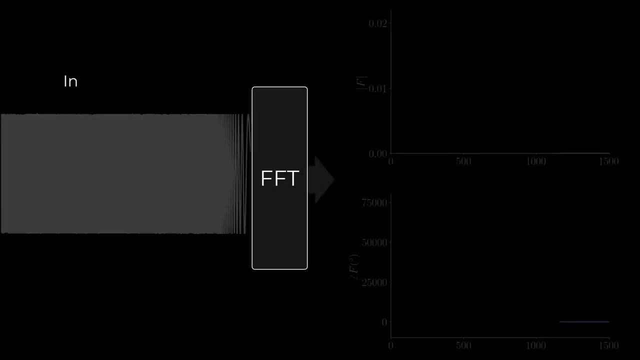 The output signal shows gradually increasing attenuation. Plotting both signals together illustrates this nicely. It's just a few lines of code to compute the fast Fourier transforms, commonly called FFTs, of these discrete time signals. The input chirp signal covers a broad range of input frequencies. 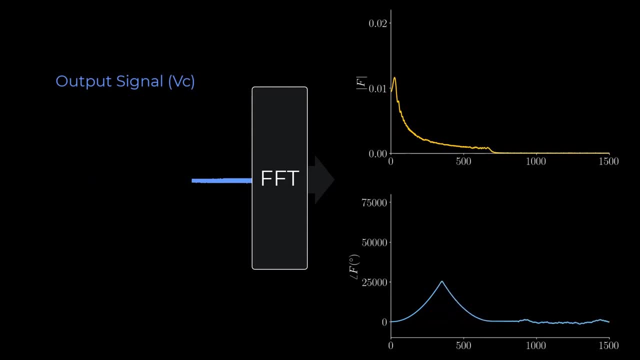 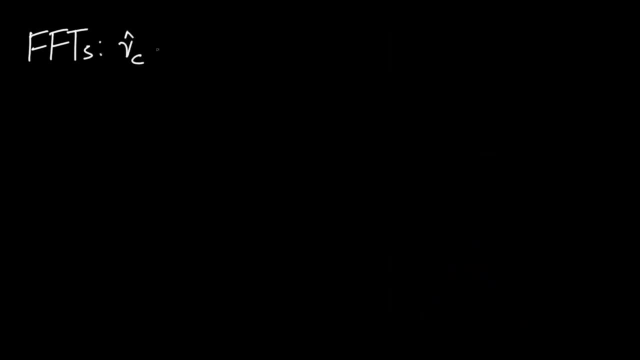 The output signal has a similar frequency range but has been modified by the RC filter. If we take the ratio of the output Fourier transform to the input, we obtain the same result as the transfer function frequency response. If we compute the phase and gain of this ratio, we'll have the Bode plot, phase and gain curves.